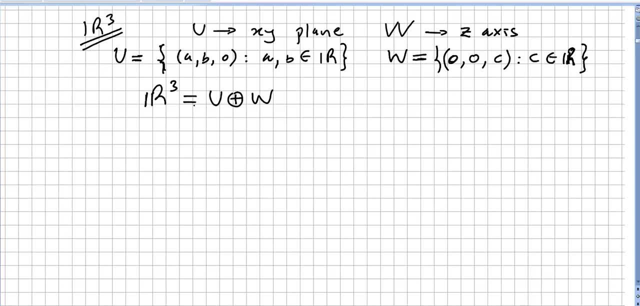 So let us see if R3 is a direct sum of our u and 0. W. Okay, so we pick an arbitrary vector in R3, okay, so it will have this form and every single vector of R3 can be written in a unique way as a sum. 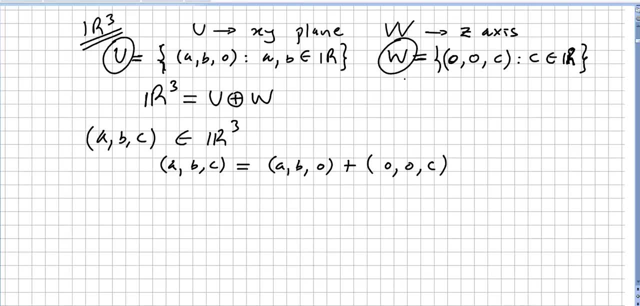 Let us say that a is the actual number of vectors in U and vectors in W. Okay, so 1, and 2, the intersection of U and W. Well, the only vector that is in the intersection of U and W is the vector 0, 0, 0. Right, That is the vector 0, 0, 0.. I have to do that. I have to do that. Let us say: if I write a new value, I write a new vector. No, I do not write a new value. 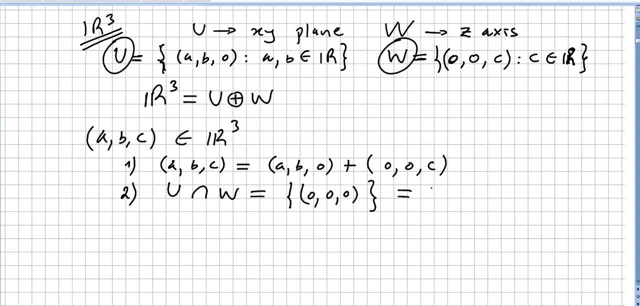 And that is not the case. Actually, I do not write any value, I write one value, I draw a new value Right. So the intersection is only zero. So we can say that R3 is a direct sum of subspaces U and W. 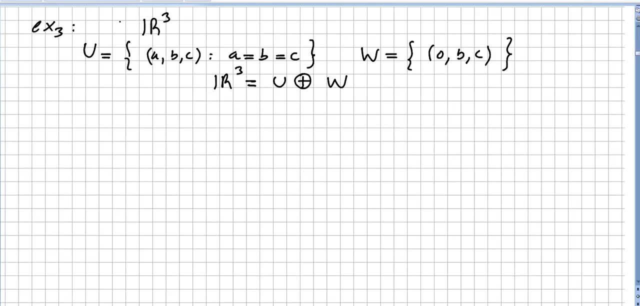 OK, yet another example. We pick the vector space R3.. And let us see if R3 can be written as a direct sum of subspaces U and W, where U is the subspace with vectors A, B and C, where A is equal to B and is equal to C. 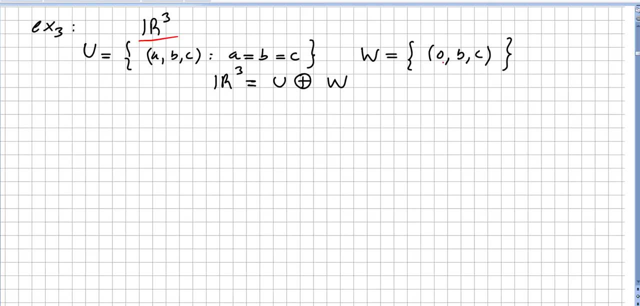 and W is the vectors 0, B C. So 0, B C. this is the YZ plane. OK, so if we pick U, intersection W, so A, B, C will be vector 0, right. 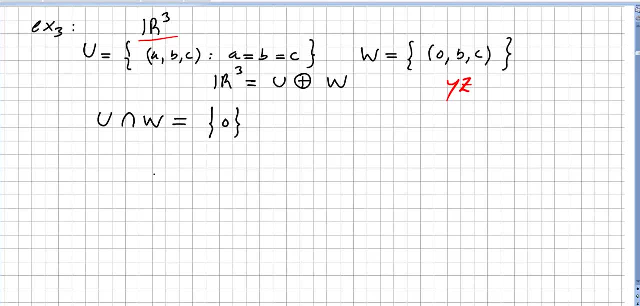 Because if we pick a vector- V, V, A, B, C- and if this vector is in the intersection, that means that A has to be equal to B and equal to C. And do not forget here A is 0.. 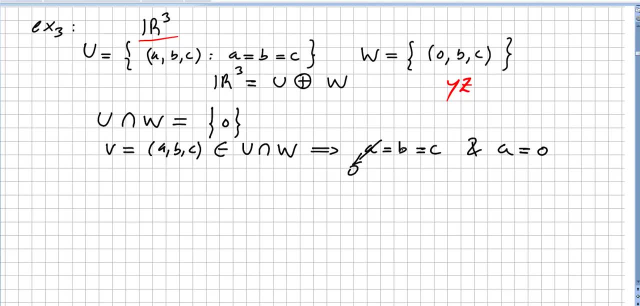 So if A is 0,, this one will be 0. So B will be equal to this one, this one will be 0, and this one will be 0, too. OK, so this means that A is 0,, B is 0, and C is 0. 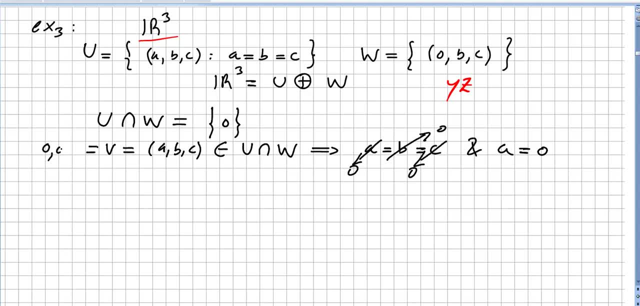 So vector V will be the vector 0, 0, 0.. OK, OK and easy to see that R3 can be written as a sum of these two subspaces. right, Because if we, If we pick a vector V but not here a vector V, let us say A, B, C, an arbitrary vector in R3. 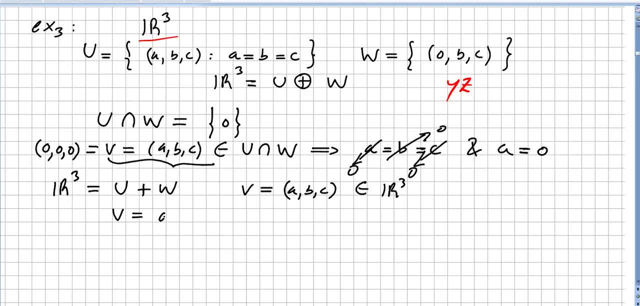 So vector V will be written as A, A, A, since these they have to be all equal plus 0, and B. OK, but what is B? B is B minus A and C minus A, right. So if we add these two vectors right, we will get A. 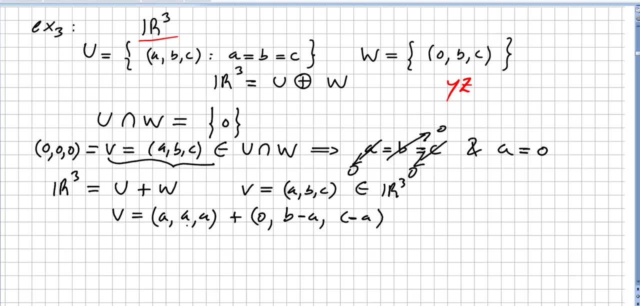 Here: A plus B minus A, we are going to get B, and then A plus C minus A, we will get C. So So both conditions- 2 is checked and 1 is checked. so yes, R3 can be written as a direct sum of these two subspaces.